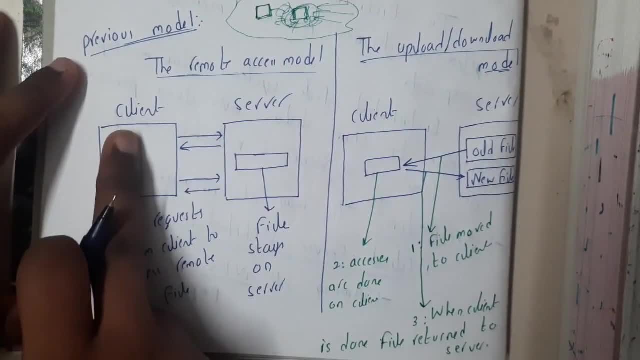 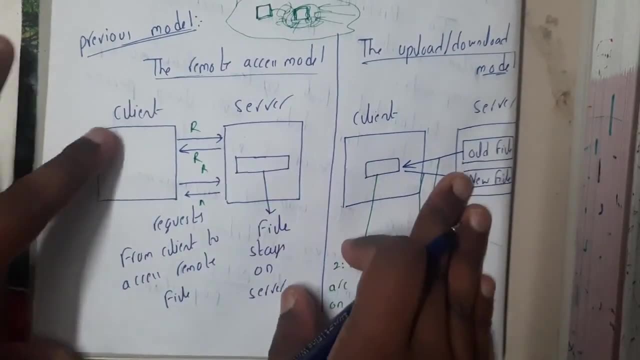 model where remote client access model, where client will be requesting for something and the server will be responding for something. Okay, So that is nothing but your previous model. And similarly we are having upload and download model also, whereas the server can download or he can. 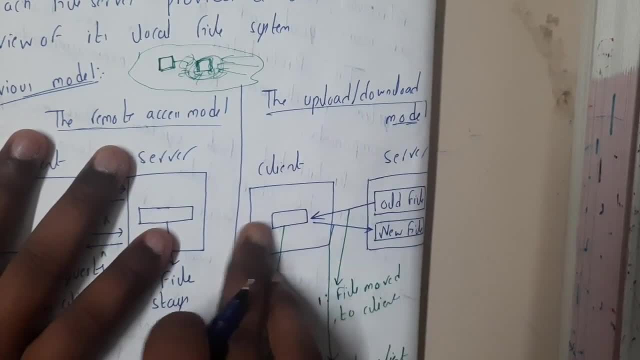 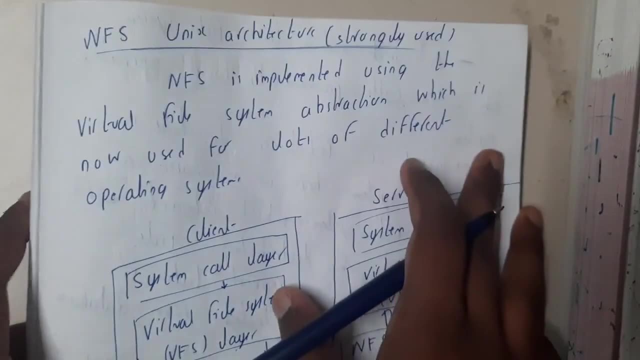 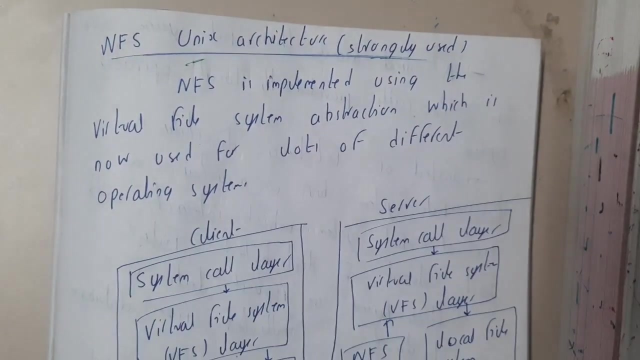 request for request for files and he can re-upload the file. So that's nothing but download and upload. Okay, Yes, I wrote the same steps here. Okay So, among which all the current day, we are using this NFS Unix architecture guys. Okay So, this is a strongly used. Okay So NFS is. 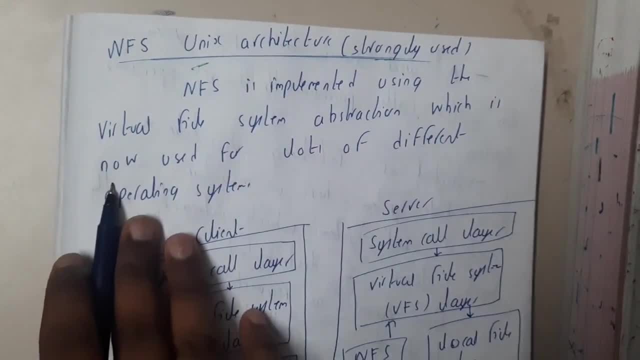 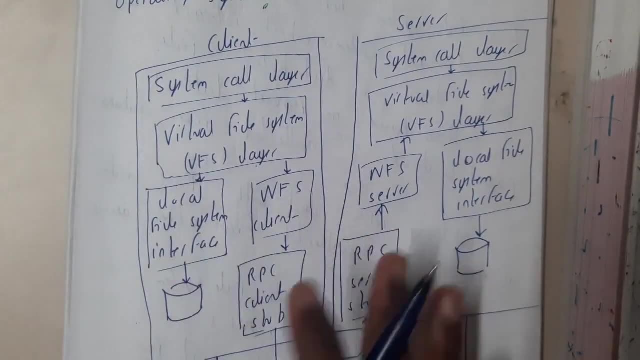 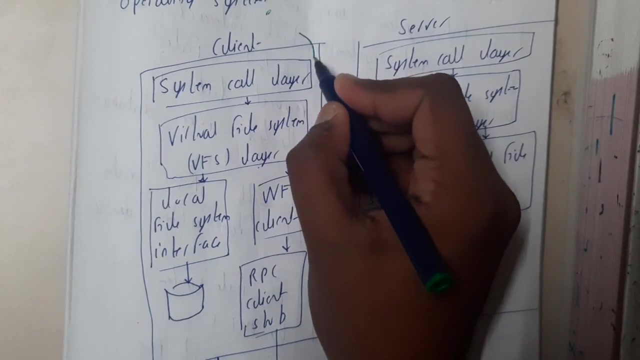 implemented using the virtual file system abstraction, which is now used for a lot of different operating systems. So it is not only for Unix guys. Most of the operating system like windows and all those are using this only okay. so we are having client and server. so basically client does some system calls. 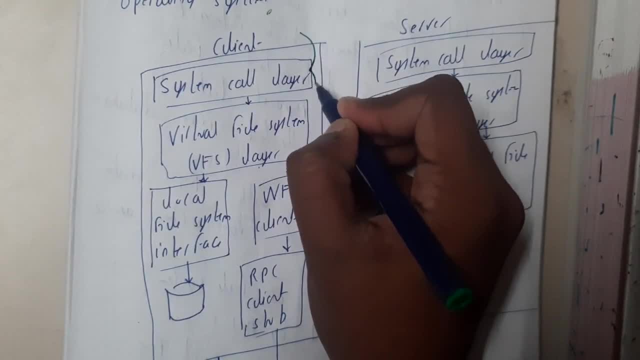 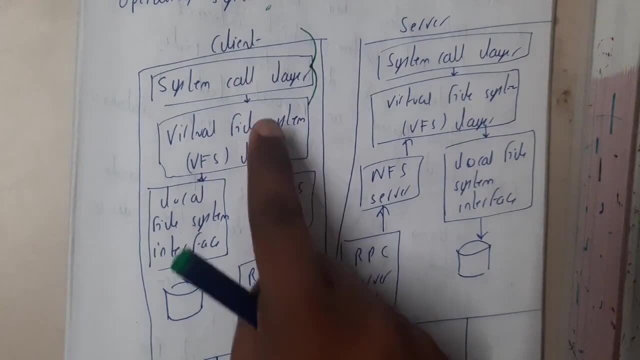 okay, and that system calls the files. whatever he is requesting will be passed to the virtual file system. so in virtual file system we will be writing the code in such a way that it will decide whether it is in the local file system or it should get from the server guys. so if it is in the local, 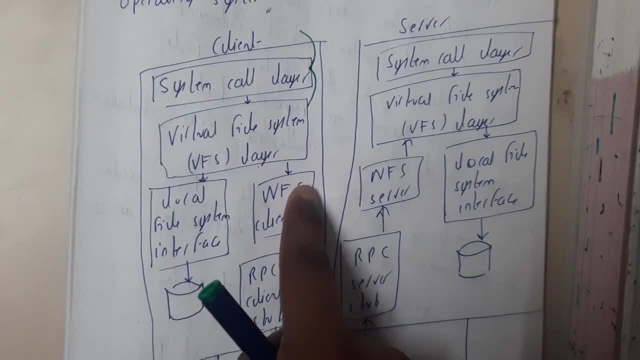 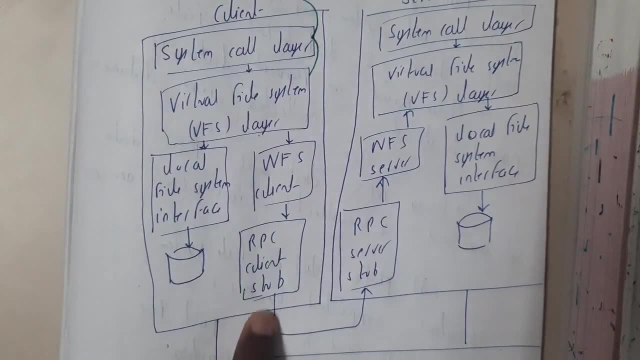 file system it will be collecting from there. else it will send it to nfs client and nfs client will be informing the remote procedure call like invoking the remote procedure call and it will send the information to the server remote procedure call and he will be requesting the nfs server and 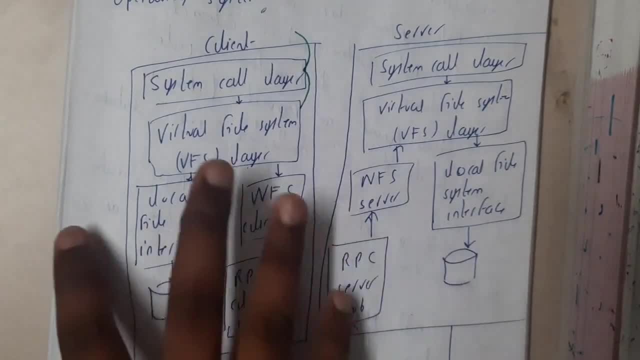 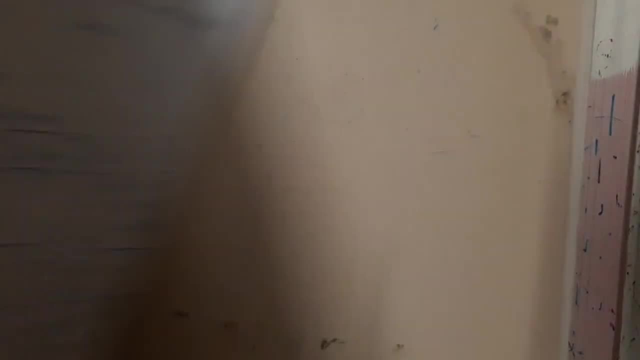 there the search will be done and from the local storage you will be getting the file. so this is the whole architecture, guys. you can just explain in your own words, guys, okay, what i explained you can write in your own words. i think i have written for this part, okay, so a client accesses the file. 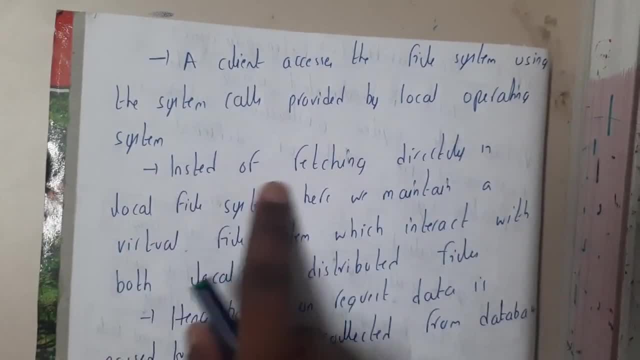 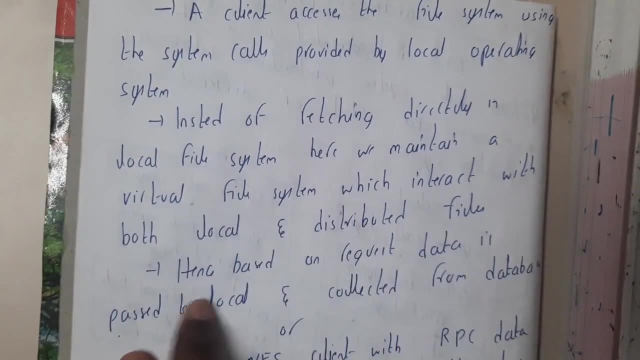 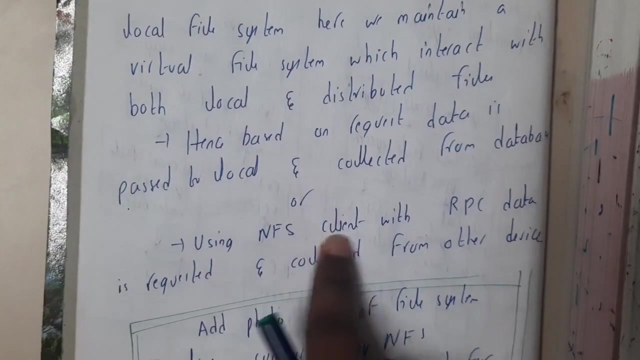 system using the system calls provided by the local operating system. instead of fetching directly in local storage, we maintain a virtual file system which interacts with the both local and distributed file system, hence, based on the request of data, pass it to local and collected from database or using nfs. 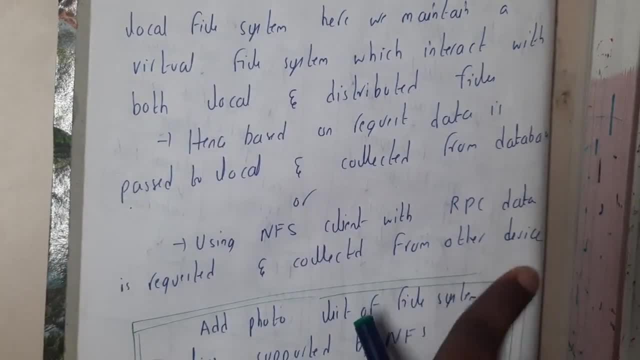 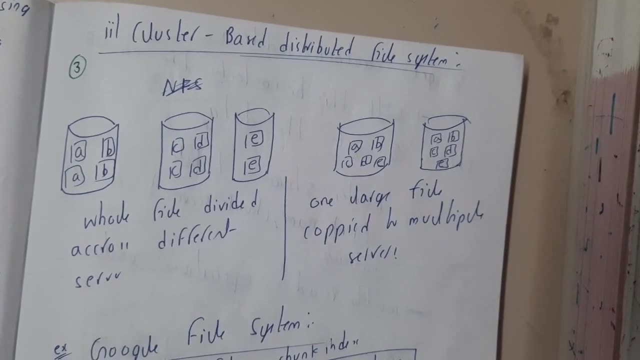 client with rpc, data is requested and collected from other devices. so this is the basic flow, guys. if you ask me, this is nfs is one of the most important topic, guys, so you might be having it out that. okay, so are there any list of operations? so these are the list of operations, guys, guys, this.